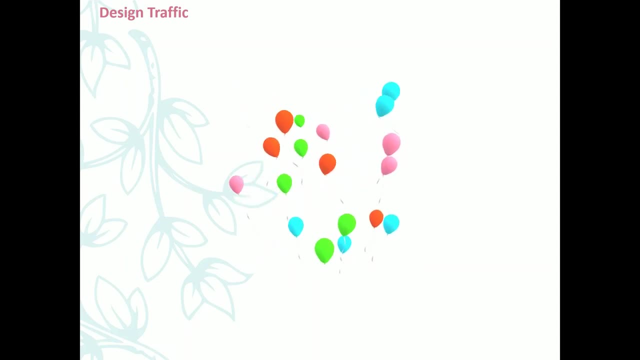 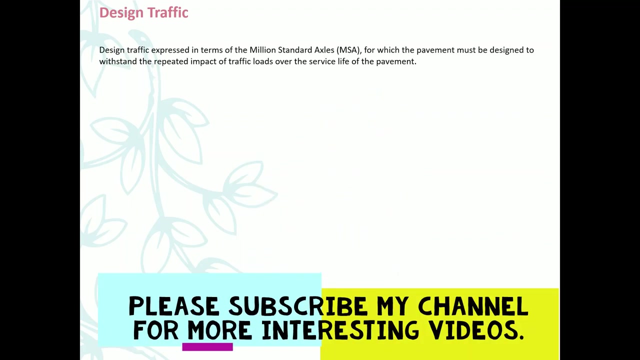 I already uploaded a video on VDF things. Please have a look over that. Then let's start Design traffic, expressed in terms of million standard axles, MSA and then, for which the pavement must be designed, Means. if you have some amount of MSA and CBR, then it can automatically get the 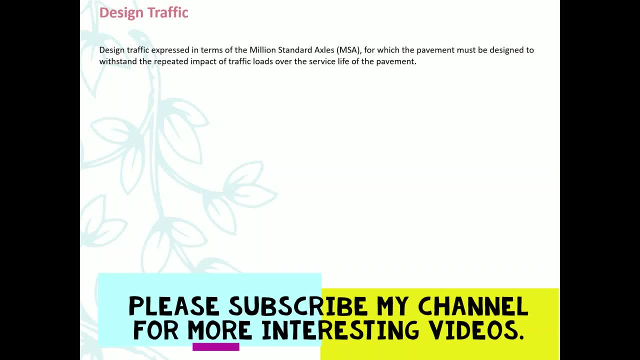 pavement thickness. So first thing is that you need to calculate the MSA, and then, from the soil samples, you will get the CBR percentage. So, based on both values, you will get the pavement thicknesses. So then, traffic loading expressed is as equivalent single axle loads, and these are dependent. 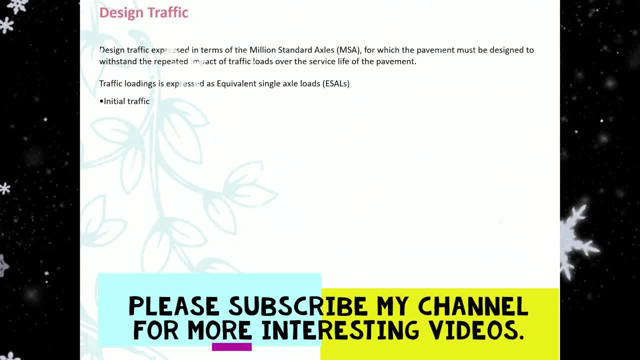 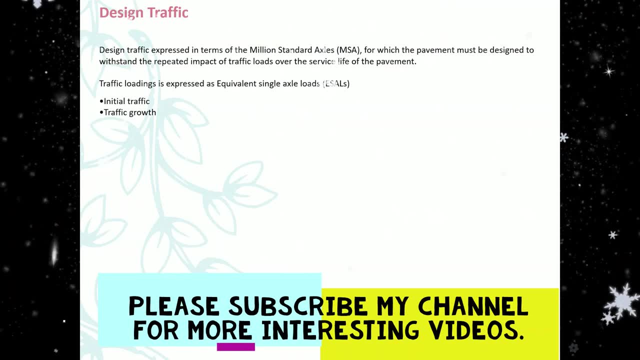 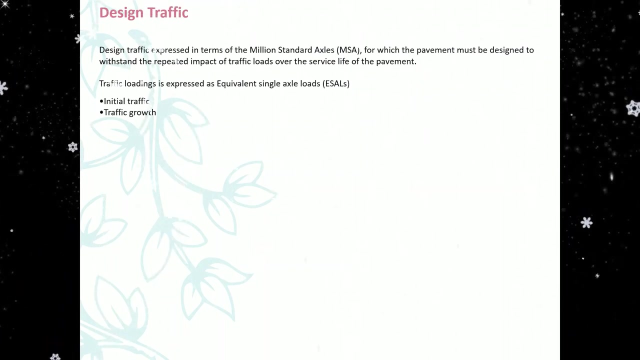 only mainly initial traffic. Whatever the initial traffic is there, That is required. the data and then traffic growth means how it will grow, Means growth rates. you have to adapt. There are two methods. are there that? for that I will keep a separate video growth rate calculations. And then number of lanes means whether it is two. 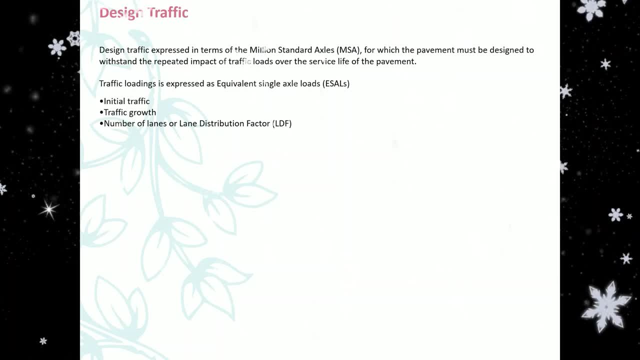 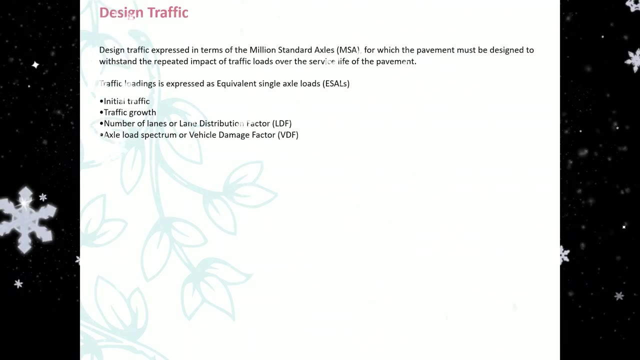 lane or dual way carriageway. that type of This is also one dependent factor. This is also one dependent factor for the MSA calculations. And then axle load, spectrum or vehicle damage factors. very, very important thing. Okay, these are the requirements for MSA calculations. 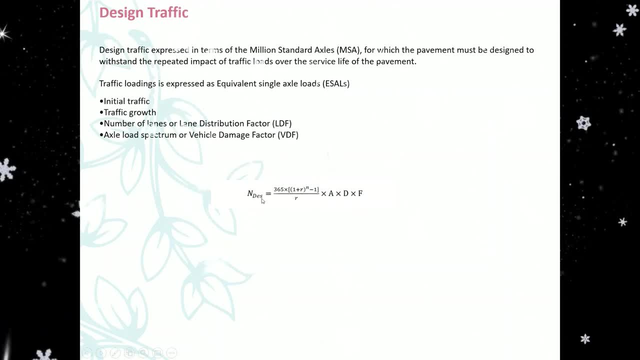 Next, this is the formula I think you must be aware in ARC 37, see: N is N design equal to 365 into 1 plus R, all power, N minus 1 by R into a, into d, into f, So where? 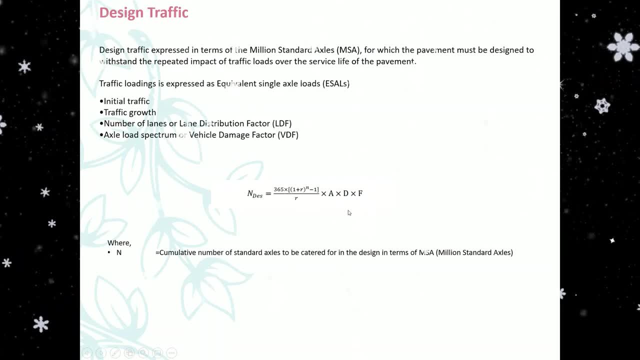 n is nothing but cumulative number of standard axle loads, that is msa, okay. and then a is initial traffic of the year of completion of construction in terms of commercial vehicles per day. okay, this calculation we are doing a different way in excel sheet. and then n is design life in years. 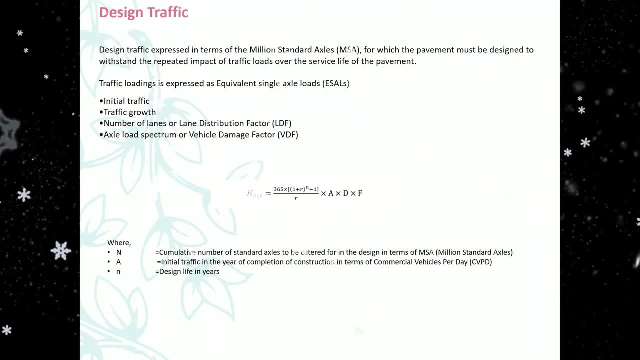 if it is flexible, 15 years, if it is rigid to 30 years, okay, and then lane distribution factor: okay, and then f- vehicle damage factor- okay. f we will get from the axle load data. d is different for the different types of carriageways: if it is dual lane carriageway and then if it is a three lane. 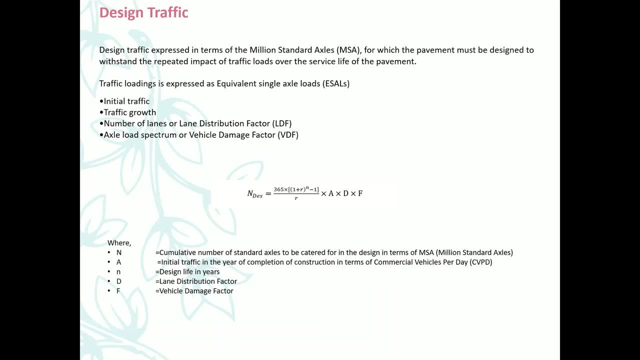 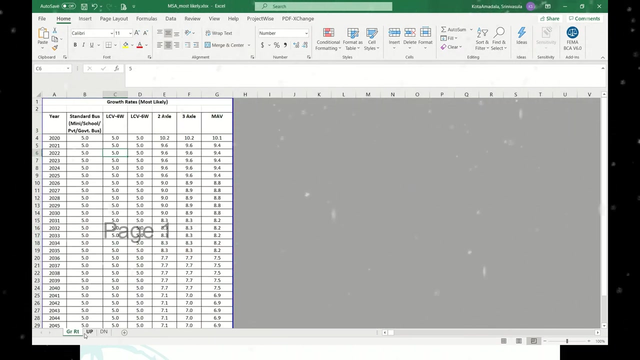 single type or four lane or single type, so it will vary actually. so in irc 37 they have mentioned clearly for what type of road what is the value. okay, paragraph 4.5. you can refer that. so now. now let's go to the excel sheet. see, in this i have three sheets. one is growth rate. 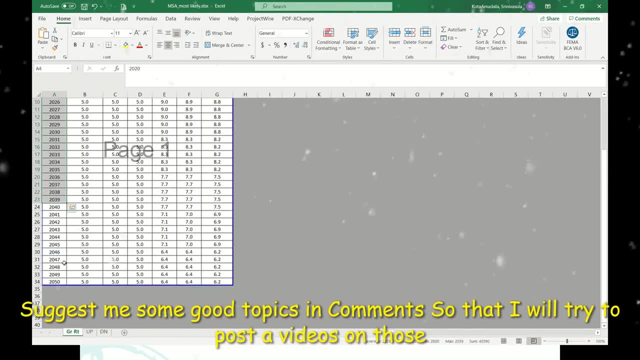 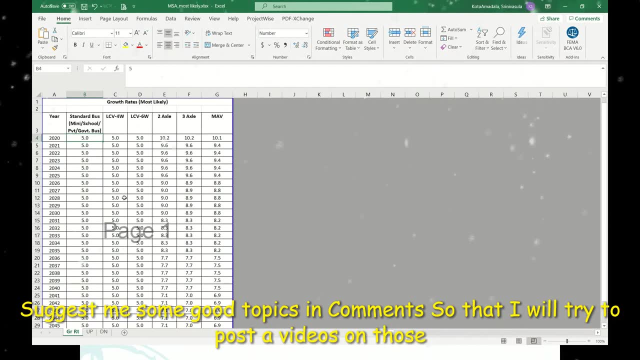 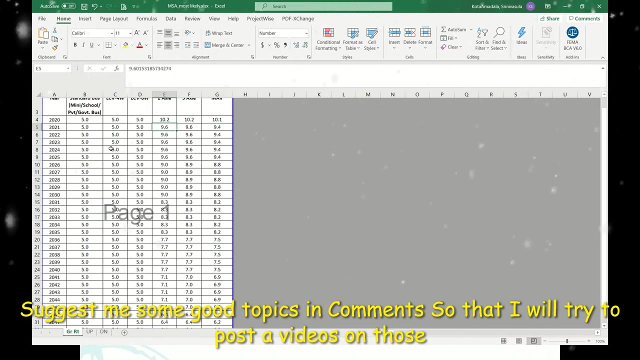 we have calculated year-wise, okay, so can you see? so buses, the growth rate we have adopted is five percent only for the all years. and then we have adopted growth rate much vary in this three categories because trucks will get increased. so 10.2, 10.2, 10.1, so remaining all are same. okay, this is the growth rate of points we adopted. 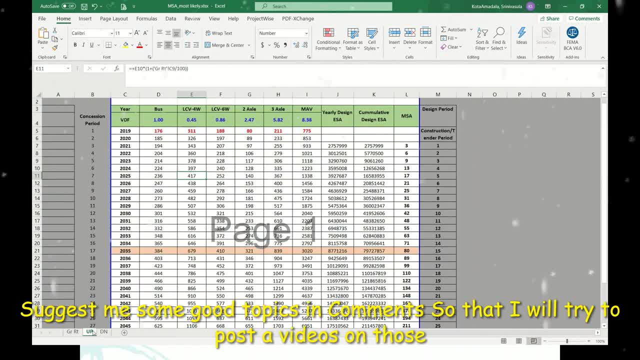 okay, then one is up for up direction, one is down direction because it is a, it is for the four lane carriageway. so we need to adopt two directions. so accordingly, we need to provide the thicknesses, because in up direction vdf values will vary. in down direction, vdfs will vary. 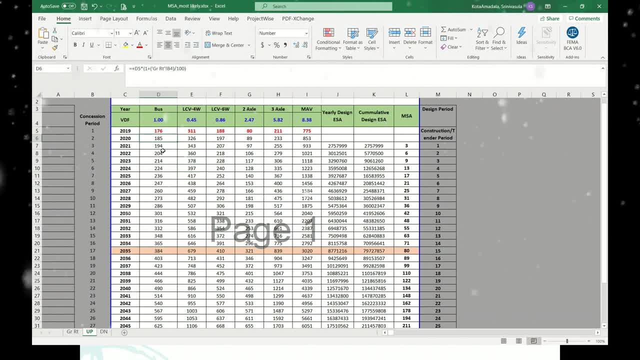 so we have to calculate separately. so let's start here. so what are the types of vehicles you need to take? the same as we have taken for vdf calculations. so buses- lcv. four-wheeler, lcv- six-wheeler, two-axle, three-axle, multi-axle. 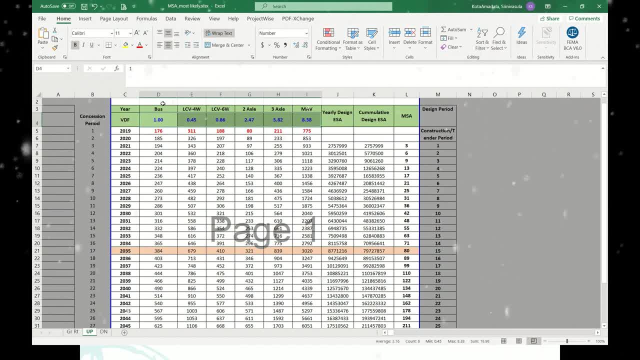 vehicle. okay, so these are the vdf values, what we have calculated from the axle load data, and then this is the base year volume. this 176 is the buses, and then 311, 188, 80, 217, 75. these are the volume in the up direction. after that, what we did just simply multiplied with the growth rate. 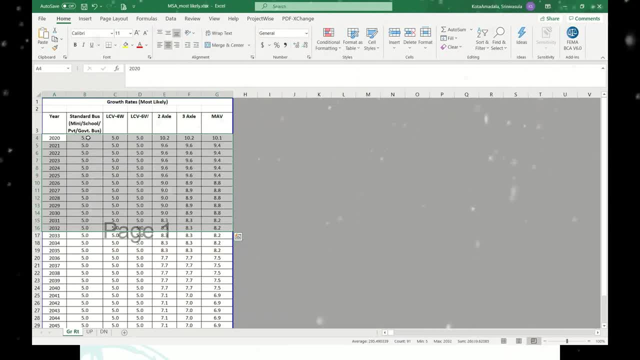 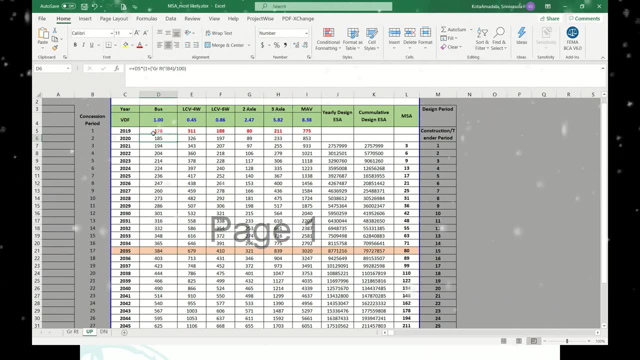 1 plus b4. is what this one five percent, five percent, that's it in a 2020, how much it will be? that is 175, five percent. we have calculated. so again, like that: 326, 197. so like this you have, we have calculated up to: 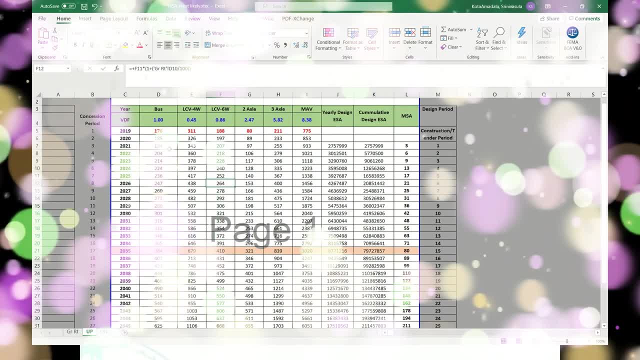 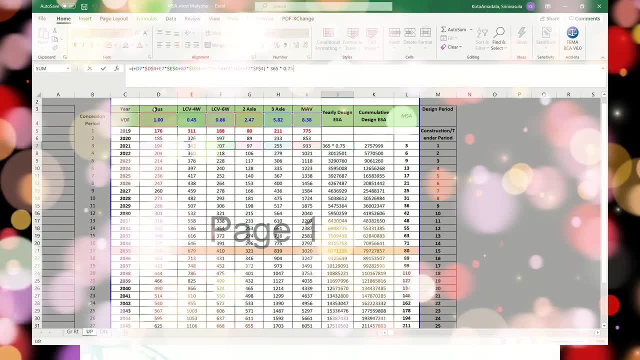 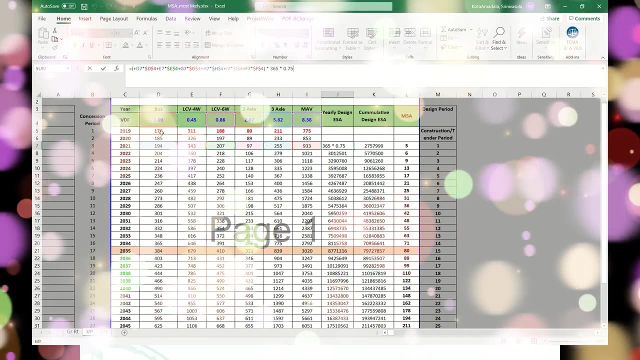 almost 30 years. okay, and then what is that yearly design? yearly design how it had calculated what i showed in the formula. the same thing, so, but here what we have, we have multiplied simultaneously with the vdf. whatever, if buses is there, so one for 194. 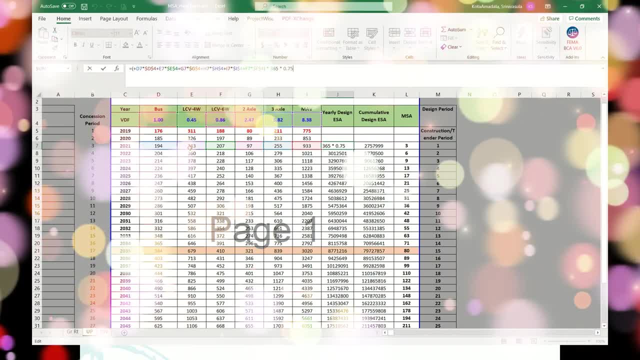 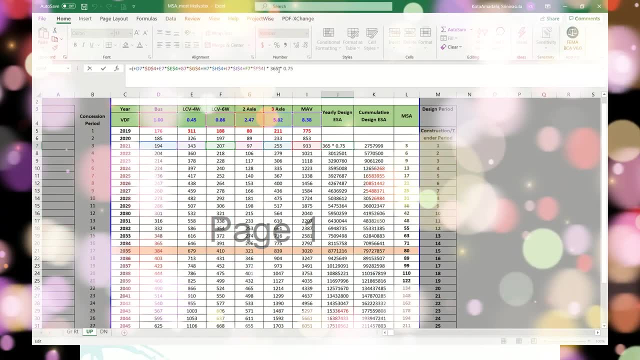 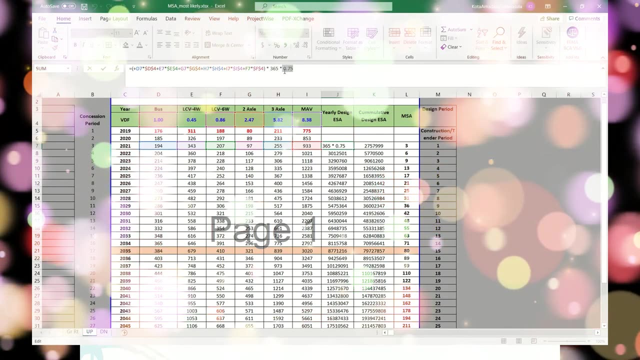 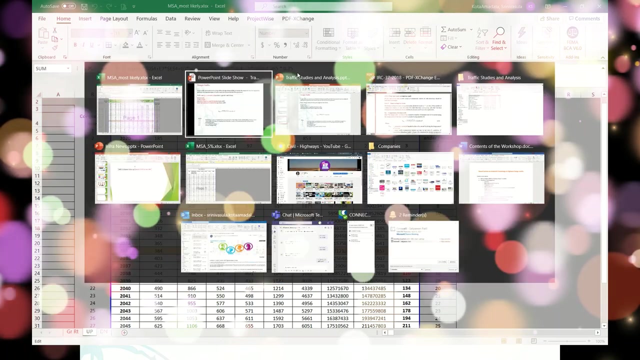 buses. what is the vdf? one is the vdf, so 343, 0.45, so like that. we have multiplied okay, then into 365, because it is yearly based, and then 0.75 is the directional distribution factor. okay, so that is sorry lane distribution factor that they have mentioned in the code, if you see. 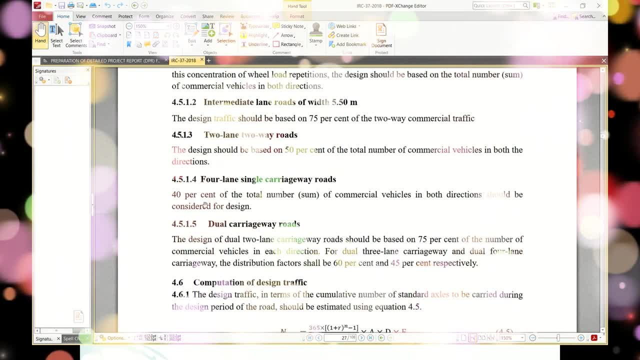 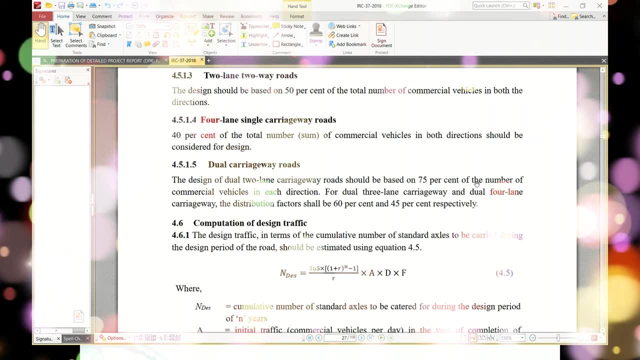 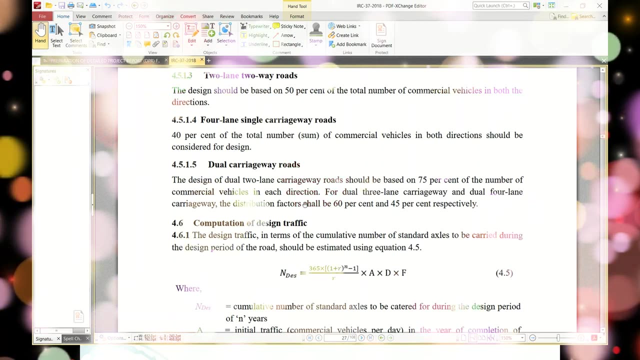 lateral distribution. okay, second, you see here competition: dual carriageway: the design of dual two-lane carriageway roads should be based on 75 percent of the number of commercial vehicles in each direction. for dual three lane carriageway, for and dual four lane carriage: the distribution. 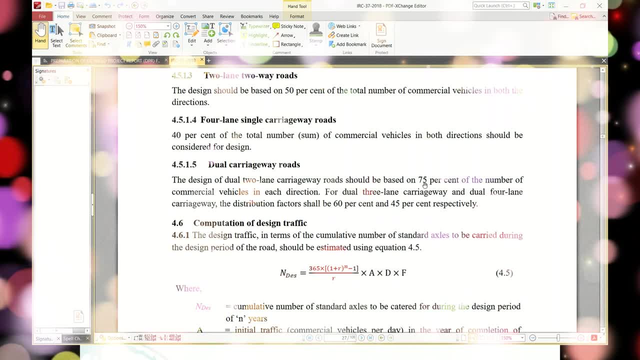 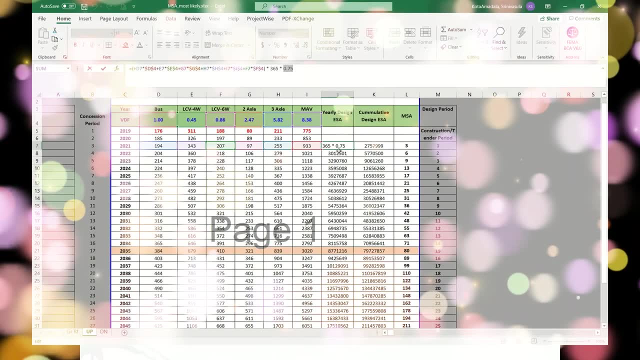 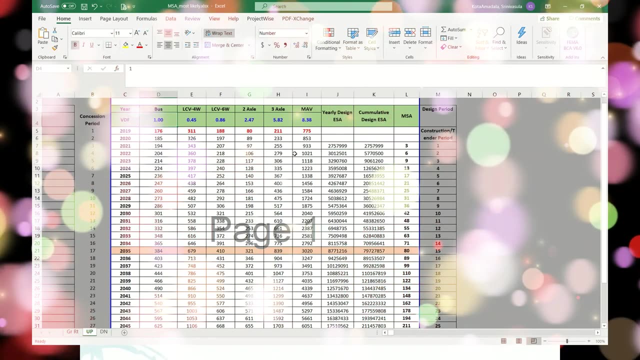 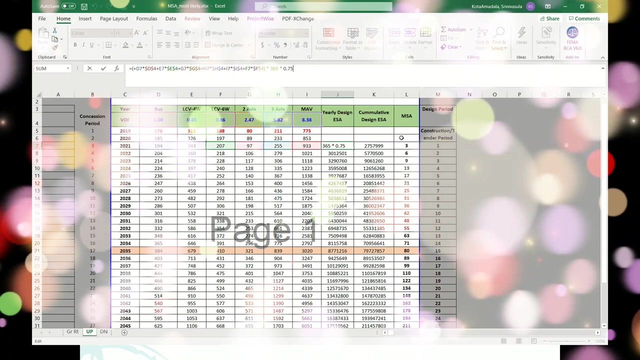 factor should be 60, 45 percent percent. hours is four length, so 75 percent. we have considered okay. so now that's why we have multiplied with the 0.75. what we did, simply, we have multiplied the traffic into pdf and then total multiplied by the 365, because it is yearly design. yes, so then 0.75. after that we have just 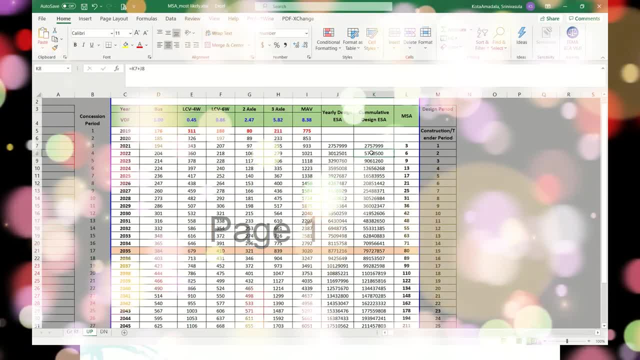 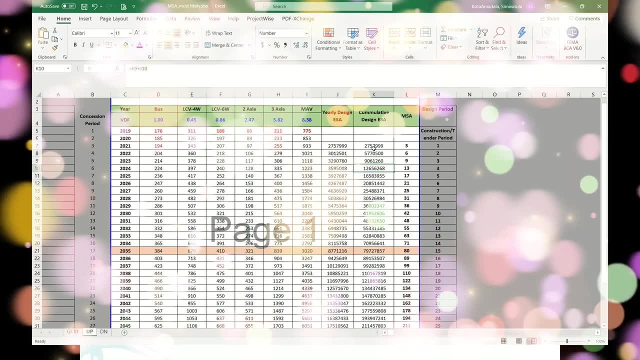 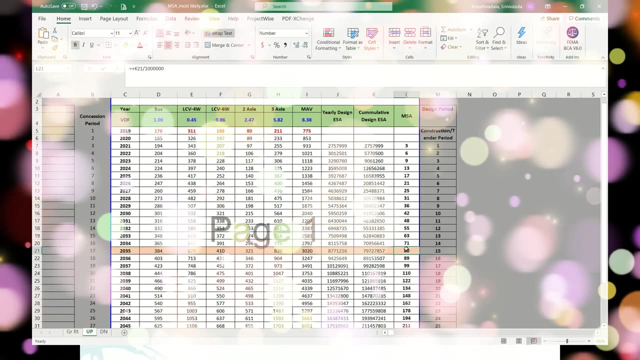 cumulated. see, here is 3 msa. then we have cumulated, just we have added the previous msa values. so like that, we have added, added, added and the at 15th year. what is the value? that is 80 msa. so this one. 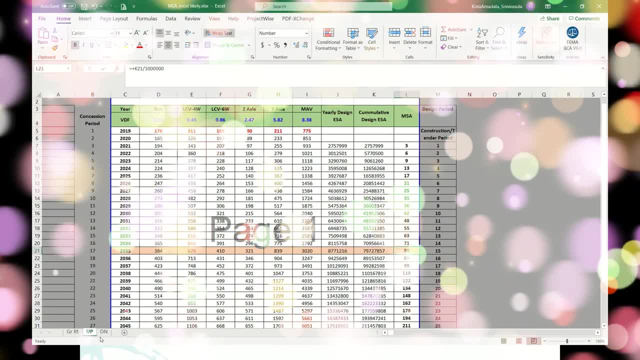 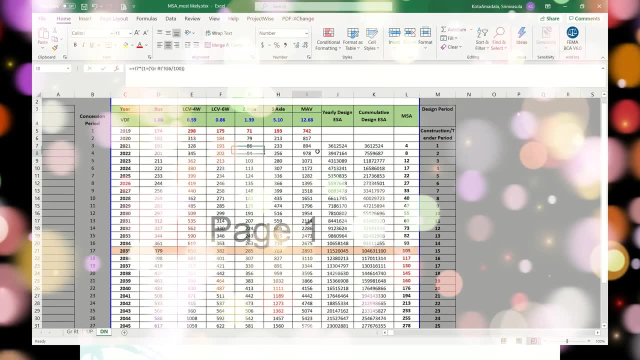 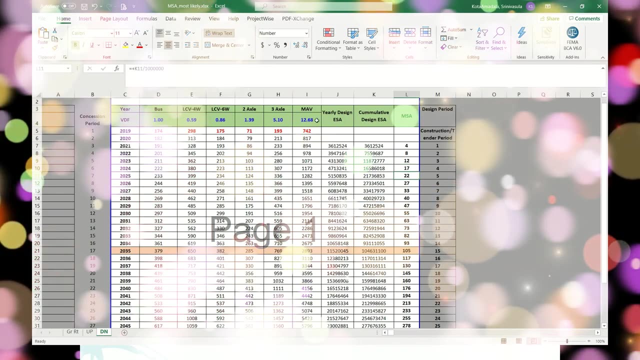 is final. this one is in a up direction. similarly. similarly, we followed for the down direction. see vehicle will, number will vary and msa. msa is getting higher. can you see 4 msa, 8, 12, 17 and the vdf helps you- also somewhat higher, can? 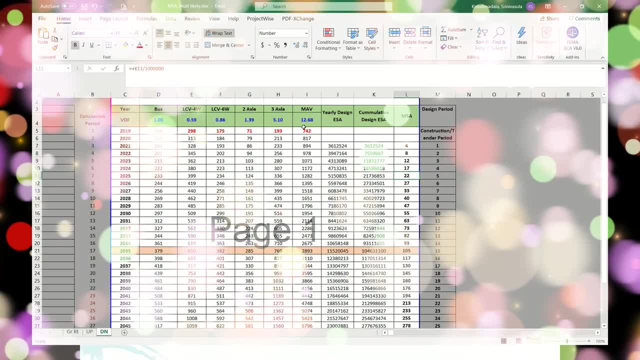 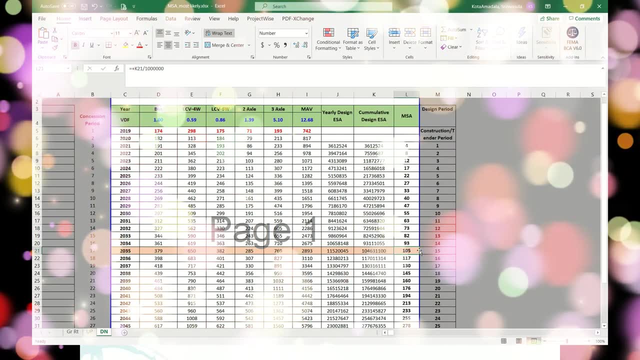 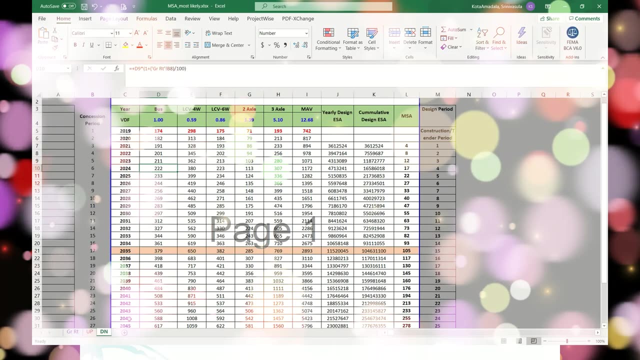 you see envio is 8.38 in up direction and 12.68 in a down direction. so in 15th year that is the msa 105. okay, so accordingly we have considered okay. so for up direction we have taken the 80 msa and 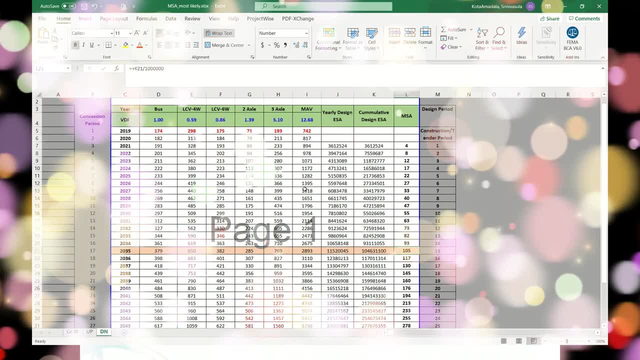 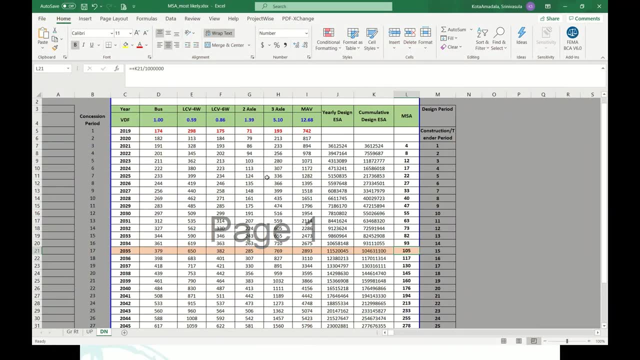 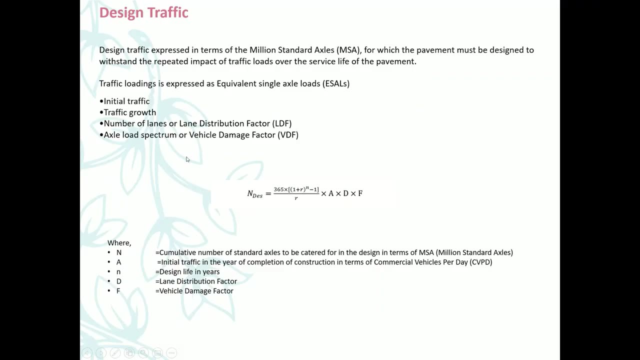 down direction. accordingly, we will provide the thicknesses also. okay, to optimize the cost. okay, that's it, guys. it is very simple. let me try to recap this. first thing we need these are the parameters. what are the parameters? initial traffic, traffic growth rates after that, lane distribution factor and. 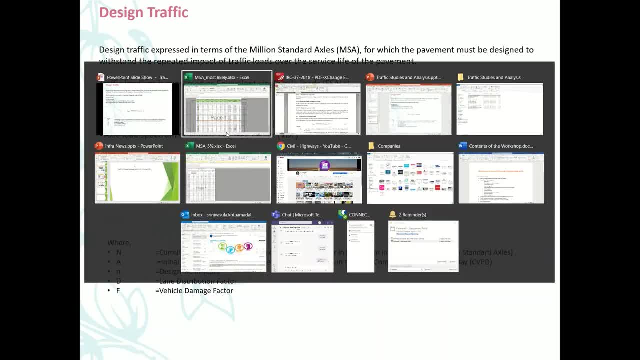 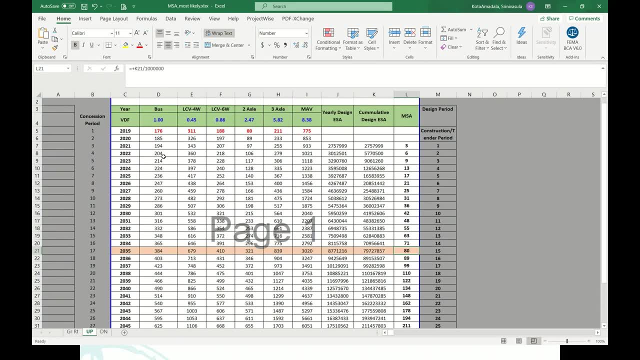 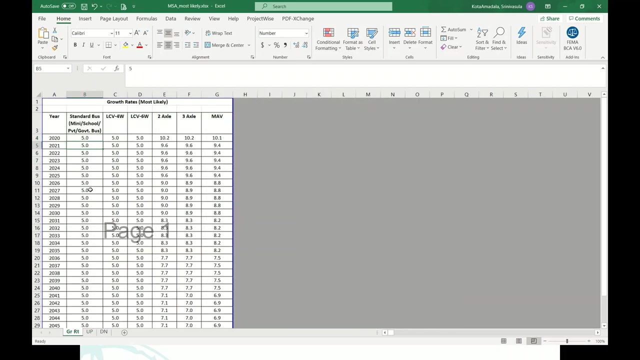 then vdf values. once we have these values, it is very easy. just growth rates, just keep it in a separate sheet and then volumes. this volumes whatever the base, base traffic volumes, and then that must be escalated to the growth rate in every year. what is that five percent growth rate? 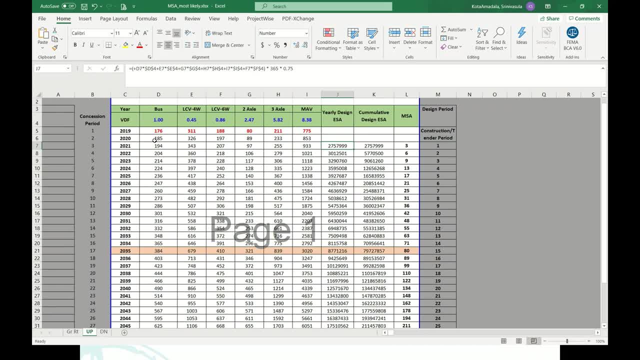 so then all these multiplied with one by one, with the vdf values, and then that must be multiplied with the 365 and to 0.75. 365 is for a year and 0.75 is for the plane distribution factor, because it is a dual plane carriageway. so